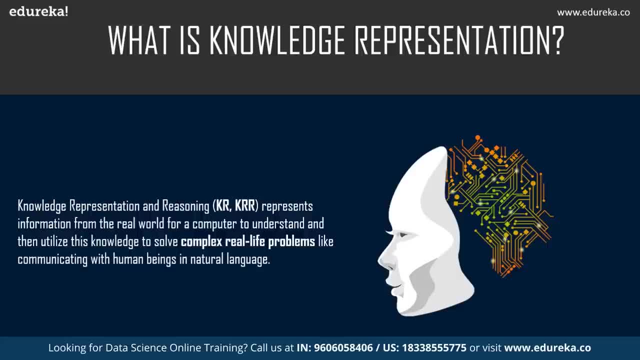 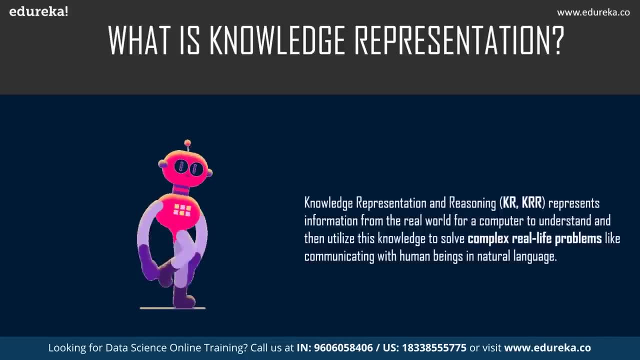 Now, one of the primary purposes of knowledge representation in AI is to be able to express the knowledge of an intelligent agent. The purpose of knowledge representation includes modeling intelligent behavior for an agent. Knowledge representation and reasoning, also known as KR or the K-RR, represents information from the real world for a computer to understand and then utilize this knowledge to solve complex real-life problems like communicating with human beings in natural language. 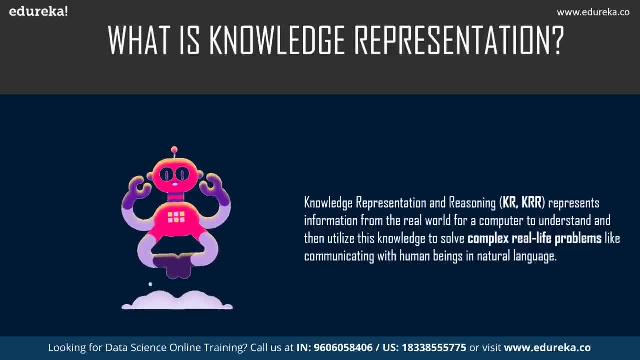 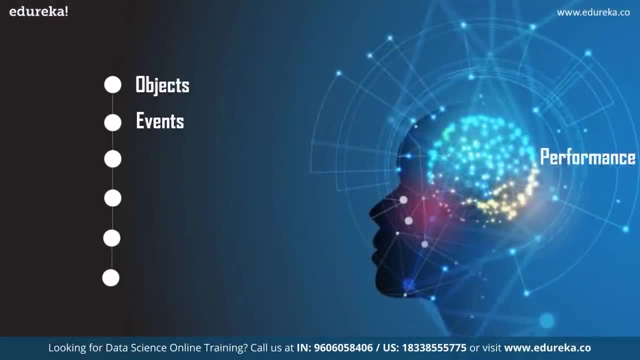 Now, knowledge representation is. AI is not just about storing data in a database- allows a machine to learn from that knowledge and behave intelligently like a human being. Now, there are different kinds of knowledge that need to be represented in AI, such as the objects, events, performance, facts. 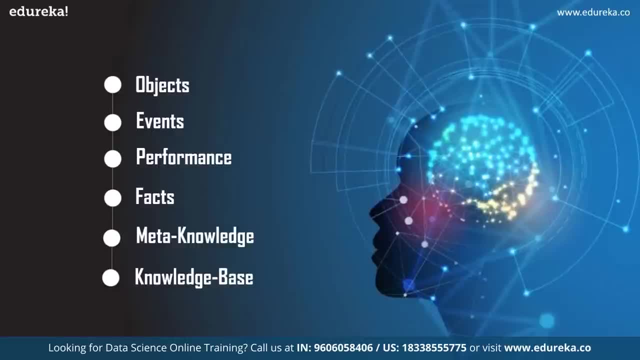 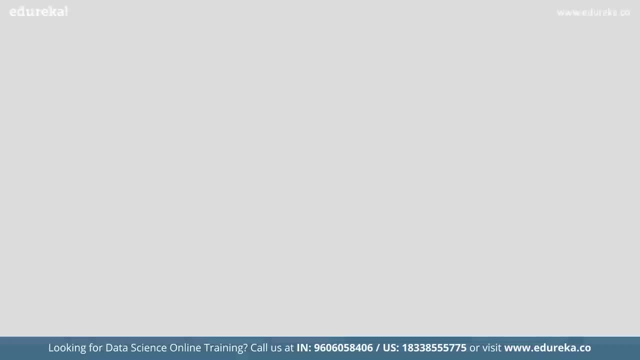 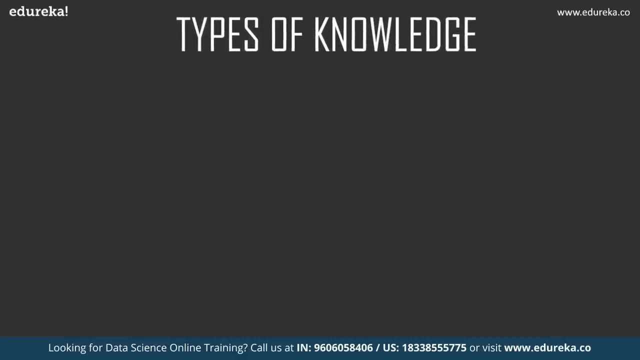 then we have meta-knowledge and the knowledge base. So these are the different kinds of knowledge that you need to represent, And now that you know about knowledge representation in AI, let's move on and know about the different types of knowledge here Now, talking about the different types of knowledge, 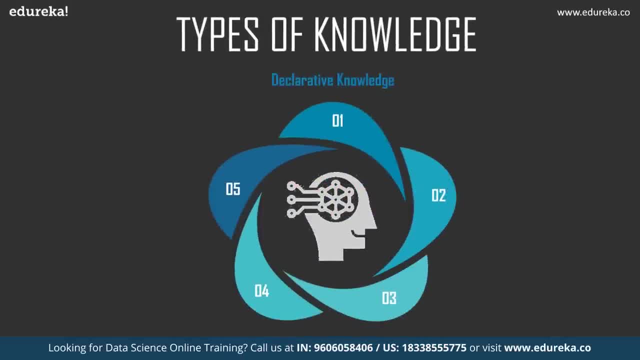 there are five types. Talking about the first one, we have declarative knowledge. Now this includes concepts, facts and objects expressed in a declarative sentence. Then we have the structural knowledge. Now it is a basic, problem-solving knowledge that describes the relationship between concepts and objects. 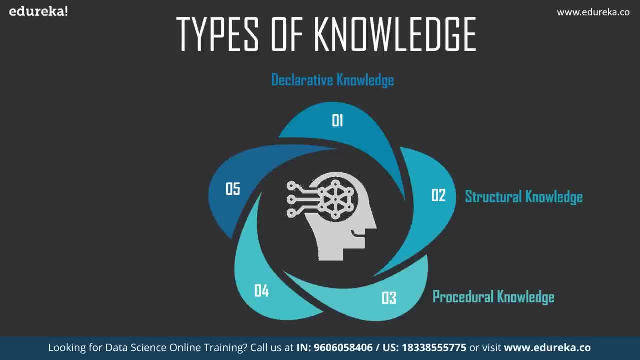 Next up, we have the procedural knowledge. Now, this is responsible for knowing how to do something and includes rules, strategies, procedures, etc. The fourth one is the meta-knowledge. Now this defines knowledge about other types of knowledge. And finally, we have the heuristic knowledge. 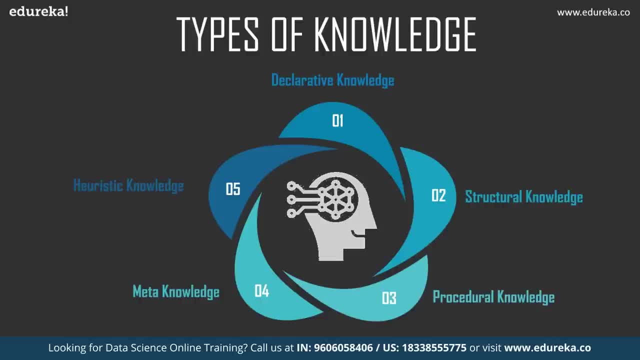 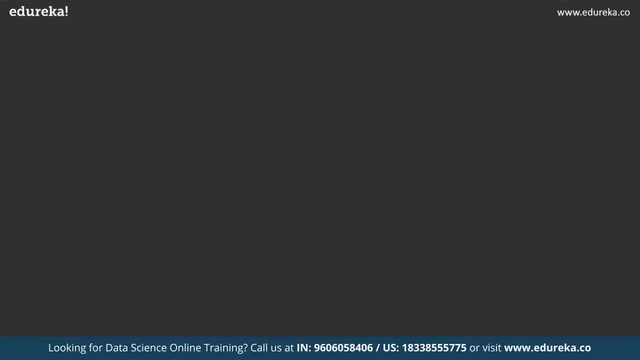 Now this one represents some expert knowledge in the field or subject. So these were the five important types of knowledge in AI. Now let's have a look at the cycle of knowledge representation and how it actually works. So, talking about the cycle of knowledge representation, 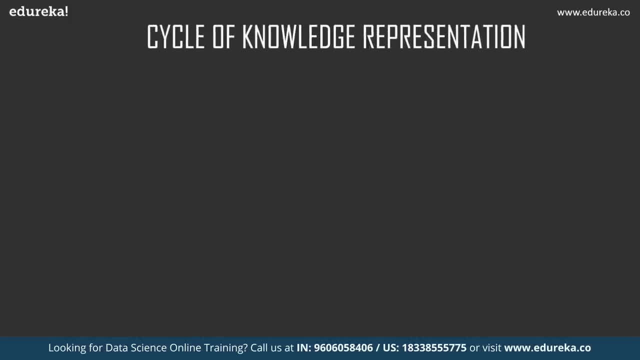 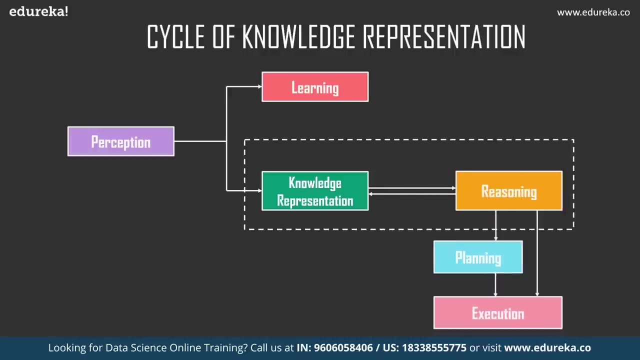 artificial intelligence systems usually consist of various components to display their intelligent behavior. Now these components include perception, learning, knowledge, representation and reasoning. Then we have planning and finally, execution. Now here is an example to show the different components of the system and how it works. 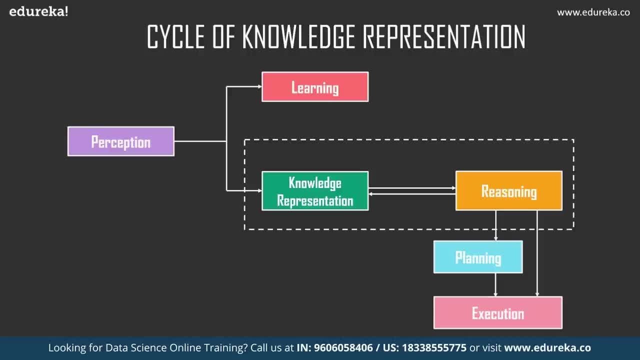 Now this diagram shows the interaction of an artificial intelligence system with the real world and the components involved in showing the intelligence. So, first of all, the perception component retrieves data or information from the environment. Now, with the help of this component, you can retrieve data from the environment. 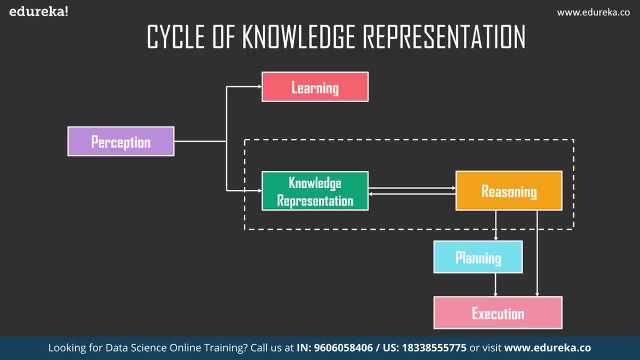 find out the source of noises and check if the AI was damaged by anything. Also, it defines how to respond when any sense has been detected. The next component is the learning component. Now this learns from the captured data by the perception component. 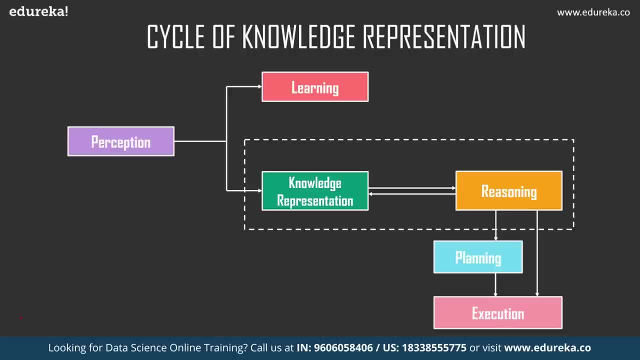 Here, the goal is to build computers that can be taught, instead of programming them. Now, learning focuses on the process of self-improvement. In order to learn new things, the system requires knowledge acquisition, inference, acquisition of heuristics, faster searches, etc. 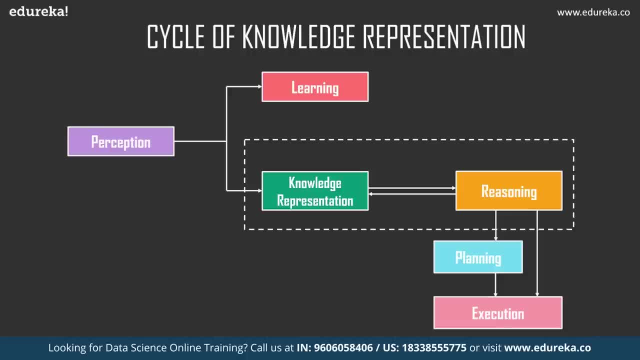 Now moving on to the next components. these are the main components in the cycle, that is, the knowledge representation and reasoning. Now this shows the human-like intelligence in the machines. Knowledge representation is all about understanding intelligence Instead of trying to understand or build brains from the bottom up. 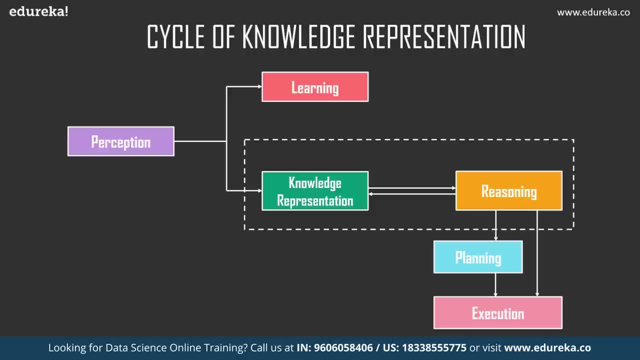 its goal is to understand and build intelligent behavior from the top down and focus on what an agent needs to know in order to behave intelligently. Also, it defines how automated reasoning procedures can make this knowledge available as needed. And finally, we have the planning and execution. 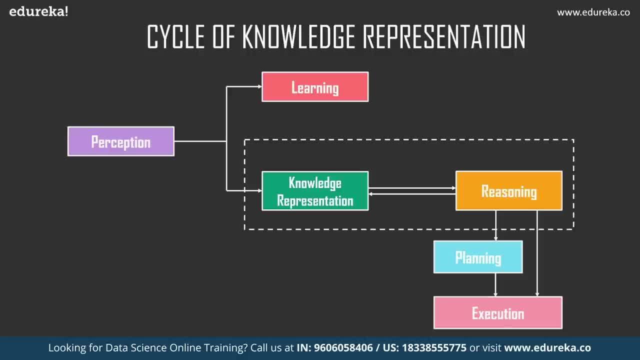 Now. these components depend on the analysis of knowledge, representation and reasoning. Here, planning includes giving an initial state, finding their preconditions and effects, and a sequence of actions to achieve a state in which a particular goal holds Now, once the planning is completed. 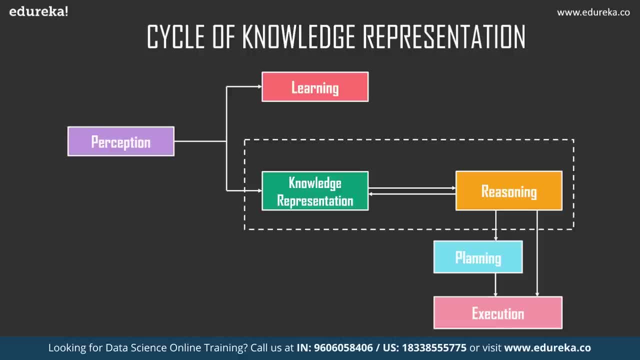 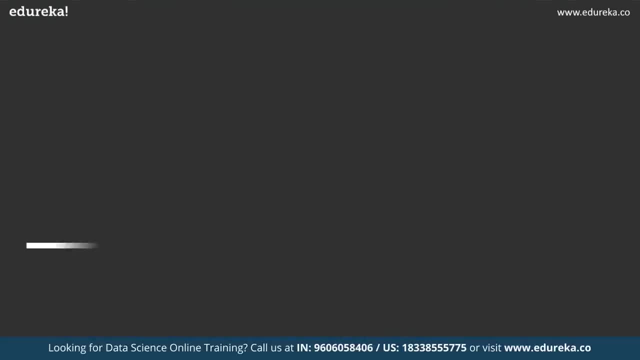 the final stage is the execution of the entire process. So this was all about the cycle of knowledge representation in artificial intelligence. Now let's move on and understand the relationship between knowledge and intelligence. So what is this relation between knowledge and intelligence? In the real world, knowledge plays a vital role. 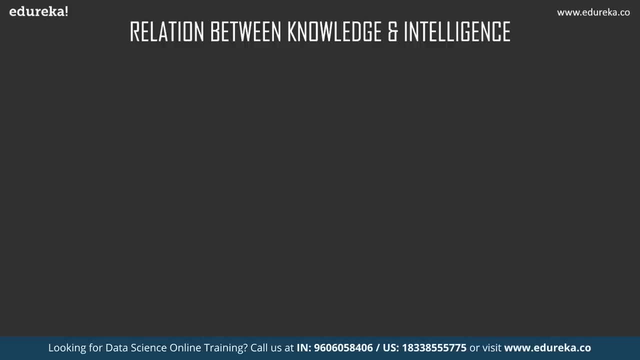 in intelligence. as well as creating artificial intelligence, It demonstrates intelligent behavior in AI agents or systems. Now it is possible for an agent or system to act accurately on some input only when it has the knowledge or experience about the input. So here is an example to understand this relationship better. 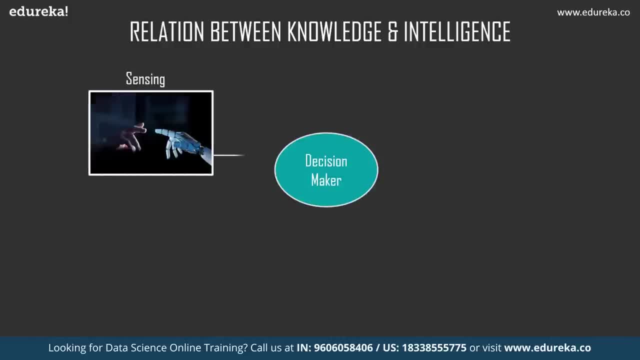 So here there is one decision maker whose actions are justified by sensing the environment and using knowledge, But if we remove this knowledge part from here, it will not be able to display any intelligent behavior. So this is the relationship between a knowledge and intelligence. 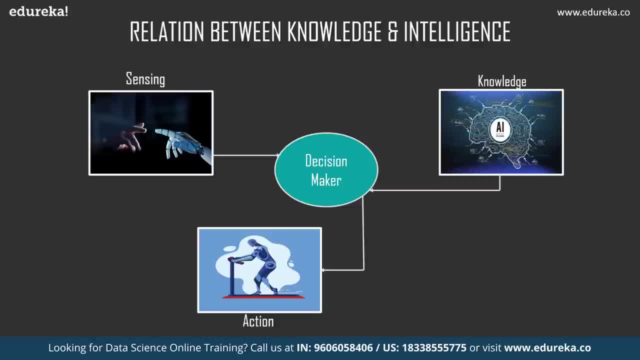 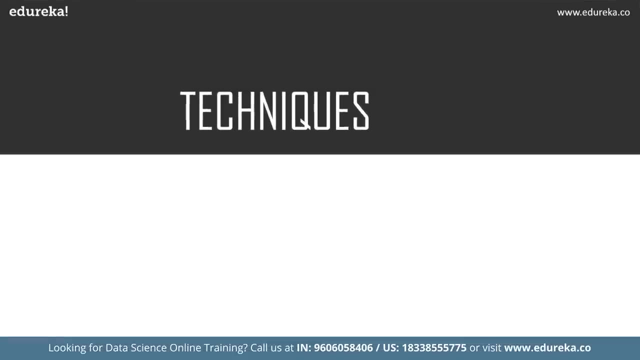 You need the knowledge in order to display any intelligent behavior, that is, for any intelligent system. You need knowledge first. So now that you know the relationship between knowledge and intelligence, let's move on to the techniques of knowledge representation in AI. Now talking about the techniques: 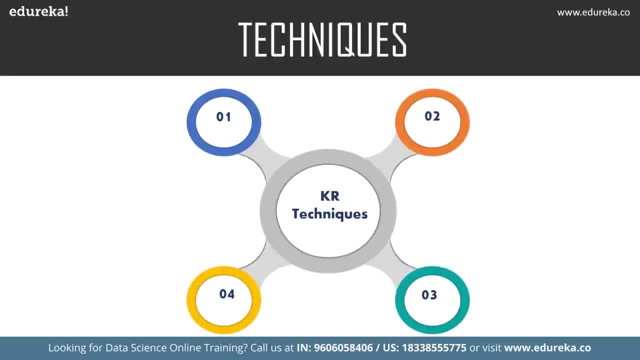 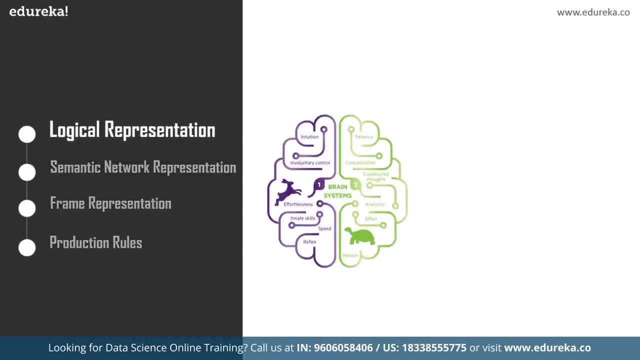 there are four techniques of representing knowledge. These four techniques include logical representation, semantic network representation, frame representation and production rules. So talking about the first one, logical representation, is a language with some definite rules which deal with propositions and has no ambiguity in representation. 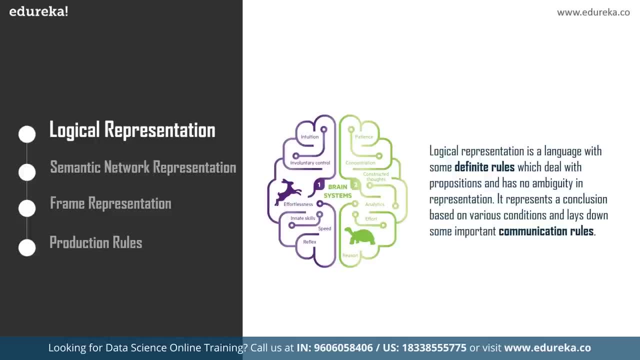 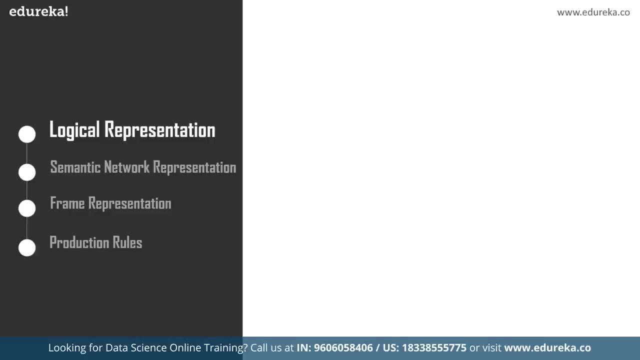 It represents a conclusion based on various conditions and lays down some important communication rules. Also, it consists of precisely defined syntax and semantics, which supports the sound inference. each sentence can be translated into logics using syntax and semantics. So what is the difference between a syntax? 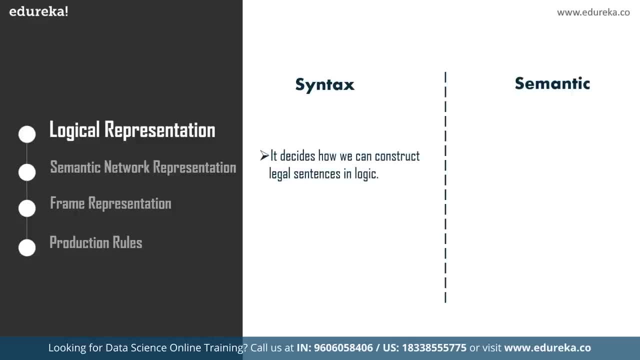 and the semantic. now for syntax. It decides how we can construct legal sentences in logic and it determines which symbol we can use in knowledge representation, Also how to write those particular symbols. but when it comes to semantics, semantics are basically the rules by which we can interpret the sentence in the logic. 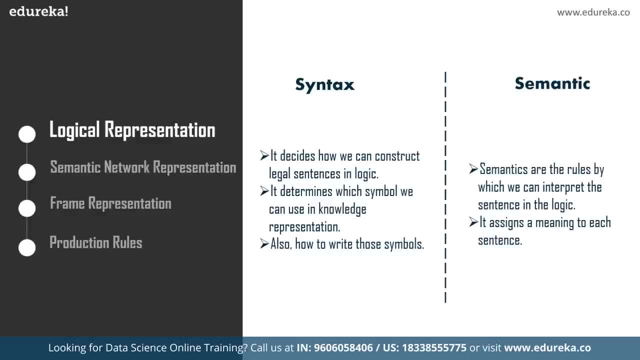 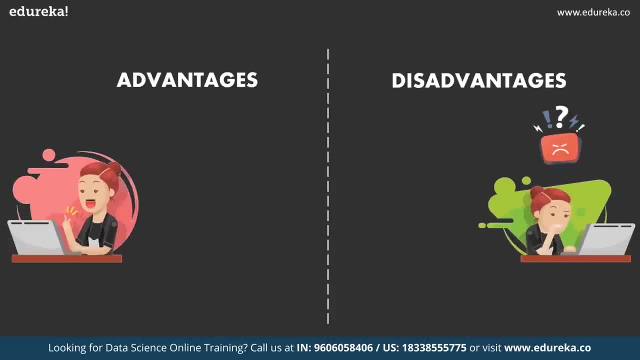 Also, it assigns a meaning to each of these sentence. So let's talk about some of the advantages and disadvantages of this representation Now. logical representation helps to perform logical reasoning. This representation is also the basis for the programming languages. These are some of the advantages of logical representation. talking 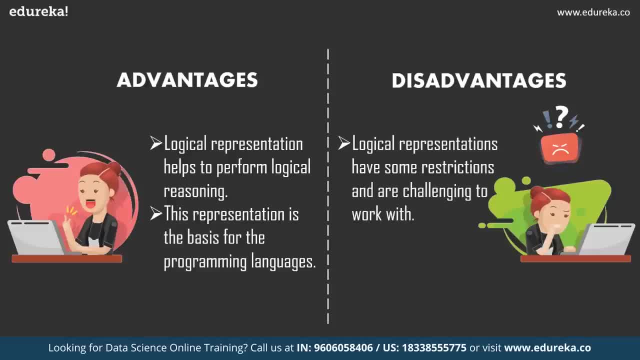 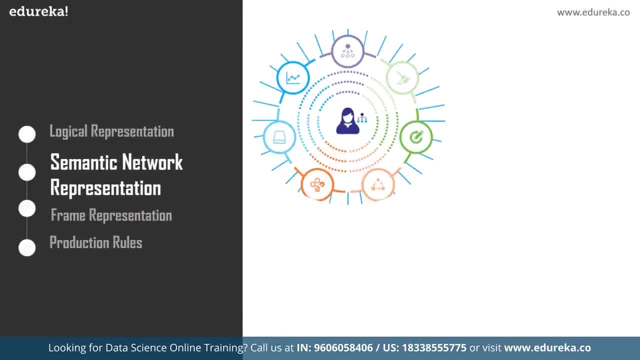 about the disadvantages: logical representations have some restrictions and are challenging To work with. now this technique may not be very natural and inference may not be very efficient. now, talking about the next technique, We have the semantic network representation. now semantic networks work as an alternative of predicate logic. 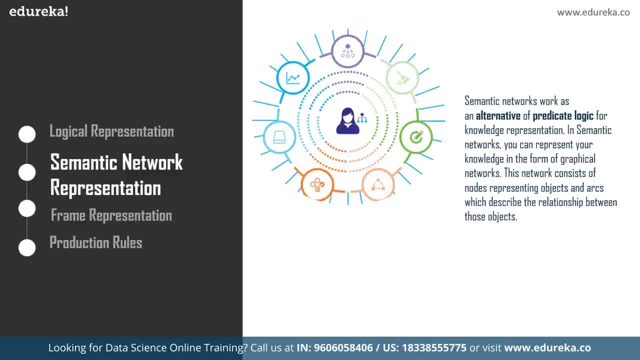 for knowledge representation. now, in semantic networks, You can represent your knowledge in the form of graphical networks. This Network consists of nodes representing objects and arcs which describe the relationship between these objects. also, it categorizes the object in different forms and links those objects. now the representation consists of two types. 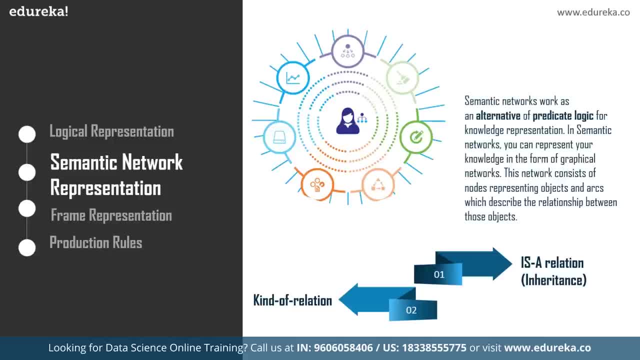 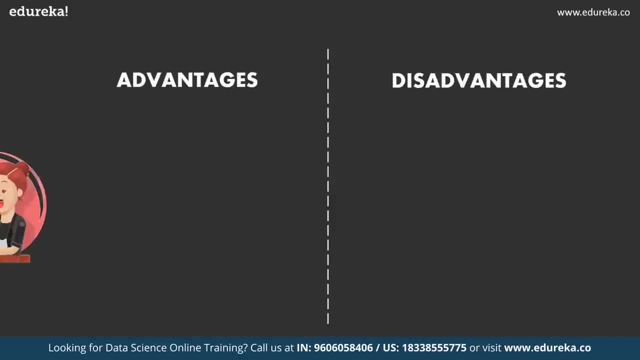 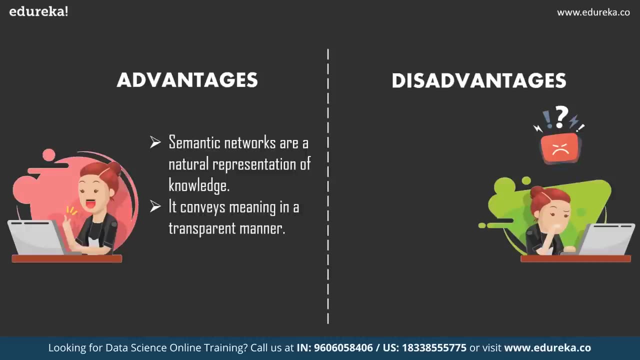 of relation. first one is an is a relationship which is also known as the inheritance, and then we have another kind of relation. now talking about some of the advantages. semantic networks are a natural representation of knowledge. It also conveys meaning in a transparent manner, and these networks are simple. 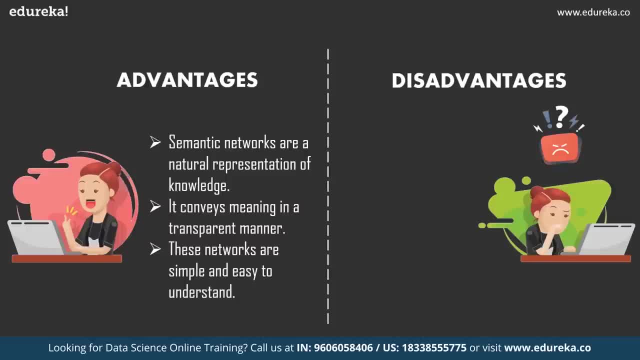 and very easy to understand. but talking about the disadvantages, semantic networks take more computational time at runtime and these are inadequate as they do not have any equivalent quantifiers. Also, these networks are not intelligent and depend on the creator of the system. So this was about the semantic network representation. 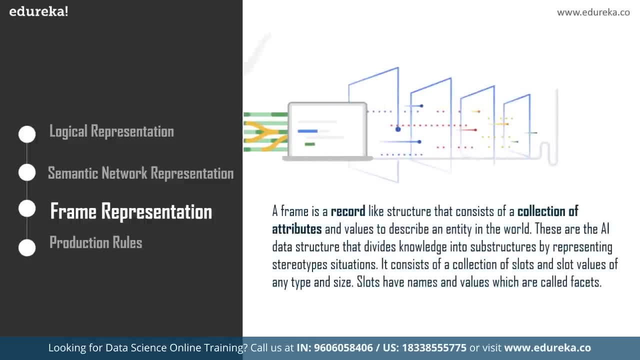 Now let's move on to the next one, which is the frame representation. now, a frame is a record-like structure that consists of a collection of attributes and values to describe an entity in the world. Now, these are the AI data structure that divides knowledge. 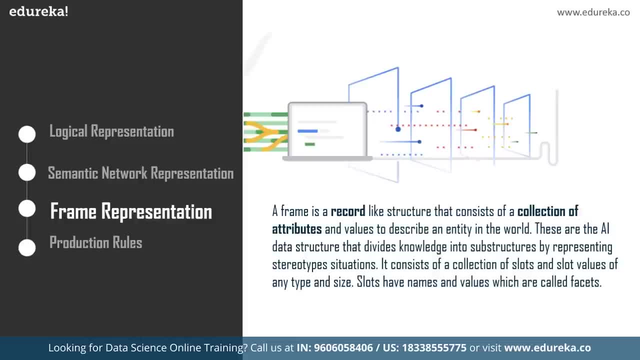 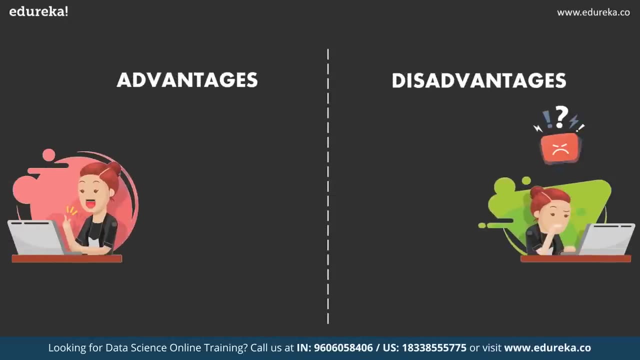 into sub structures by representing stereotype situations. Basically, it consists of a collection of slots and slot values of any type and size. slots also have names and values, which are called the facets. moving on to the advantages, It makes the programming easier by grouping the related data frame. representation is easy. 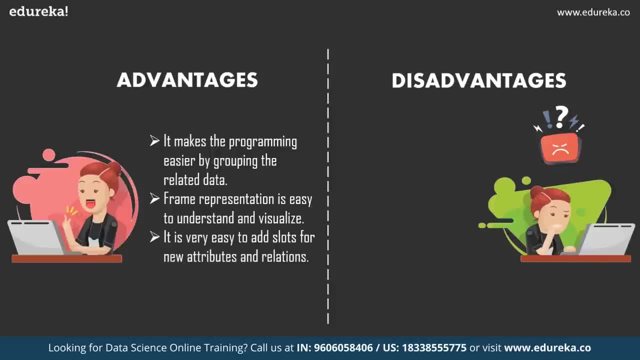 to understand and visualize. also, It is very easy to add slots for new attributes and relations. Also, it is easy to include default data and search for the missing values. talking about the disadvantages in frame system inference: the mechanism cannot be easily processed. The inference mechanism cannot be smoothly processed. 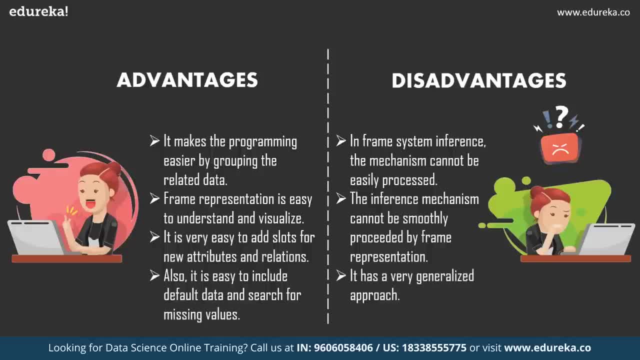 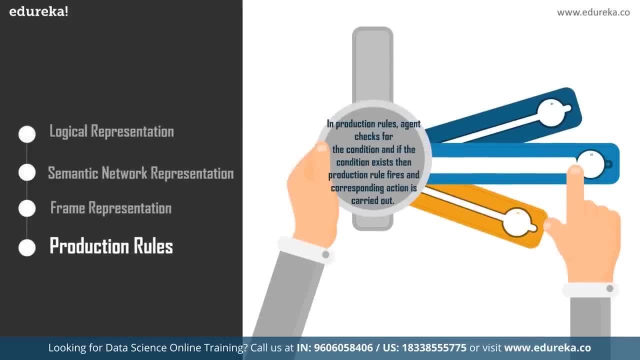 by the frame representation either. Also, it has a very generalized approach. Now, moving on to the final technique, We have the production rules. now, in production rules, agent checks for the condition and if the condition exists, then production rules fires and corresponding action is carried out. the condition part of the rule determines: 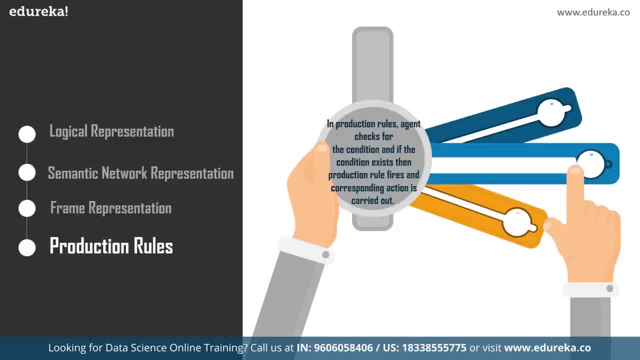 which rule may be applied to a problem, Whereas the action part carries out the associated problem-solving steps. Now this complete process is called a recognized act cycle. The production rule system consists of three main parts. The first one is definitely the set of production rules. 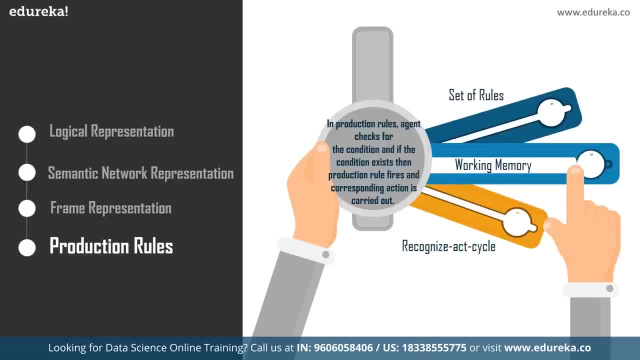 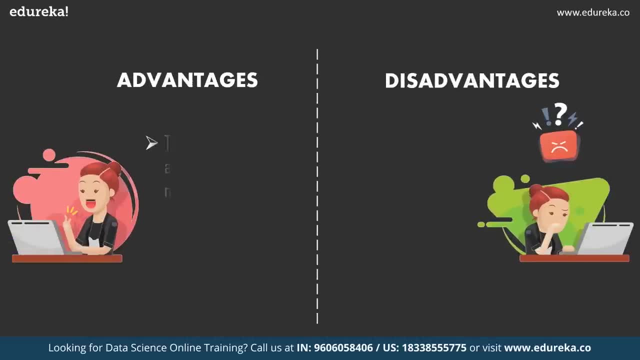 Then we have a working memory And finally the recognized act cycle. now talking about the advantages and disadvantages. first up is the advantages, where the production rules are expressed in natural language and the production rules are highly modular and can be easily removed or modified. But talking about the disadvantages, it does not exhibit any learning capabilities. 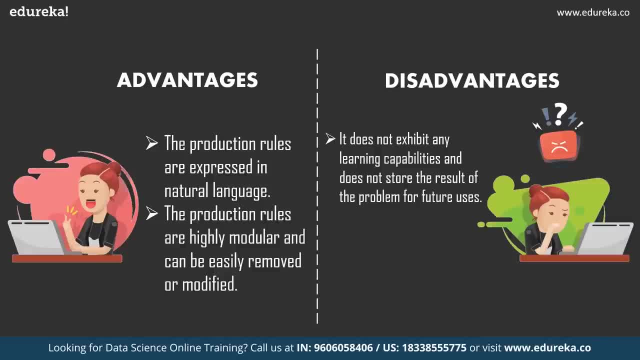 and does not store the result of the problem for future users. Now, during the execution of the program, many rules may be active does the rule-based production systems are inefficient. So these were the four important techniques for knowledge representation in AI. So now let's have a look at the requirements for these representations. 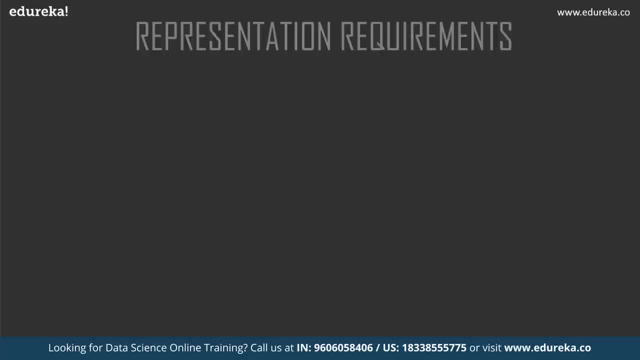 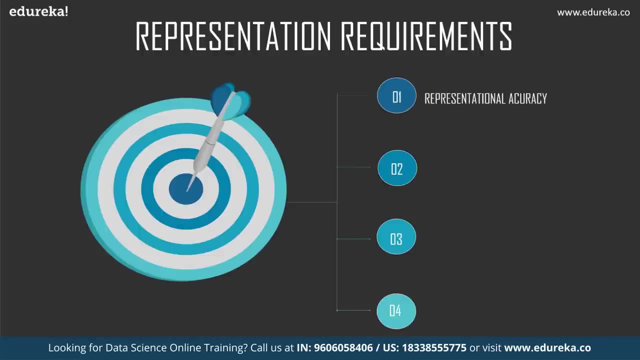 Now, a good knowledge representation system must have properties like the representational accuracy. It should represent all kinds of required knowledge. Also, it must have inferential adequacy. It should be able to manipulate the representational structures to produce new knowledge corresponding to the existing structure. 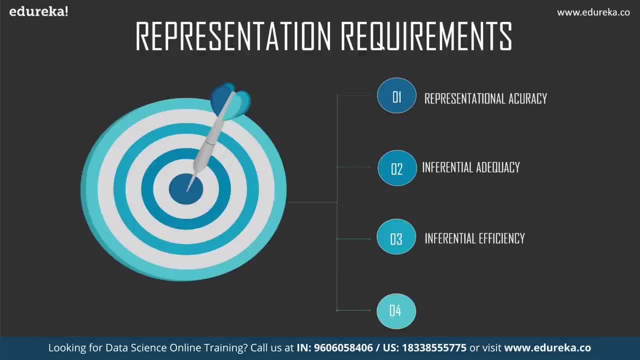 It also must have the inferential efficiency, So the ability to direct the inferential knowledge mechanism into the most productive directions by storing appropriate guides. Then, finally, it must have the acquisitional efficiency as well, That is, the ability to acquire new knowledge easily using automatic methods. 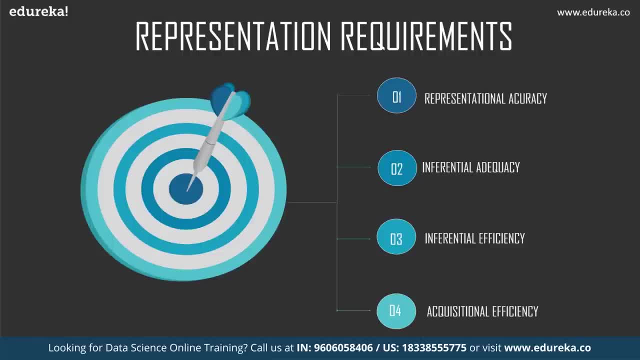 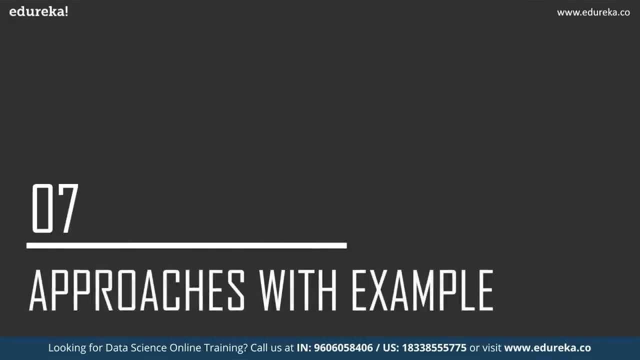 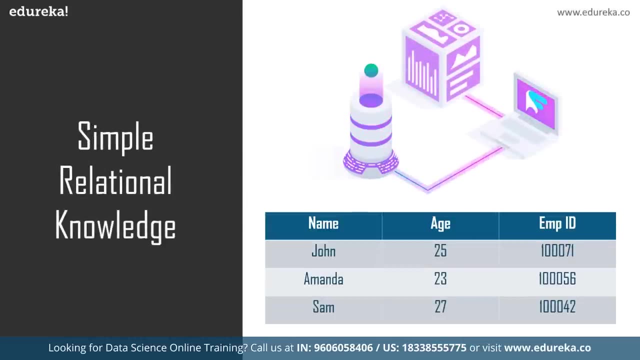 So these are some of the important requirements for the knowledge representation in AI. Now let's understand some of the approaches of this knowledge representation with examples. So the first approach is a simple relational knowledge. Now, this is the simplest way of storing facts which uses the relational method. 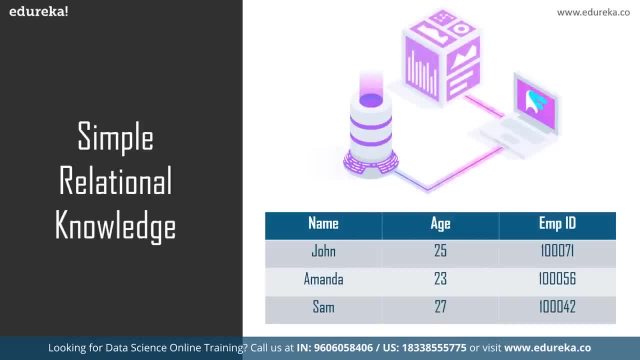 Here all the facts about a set of the object are set out systematically in columns. Also, this approach of knowledge representation is famous in database systems, where the relationship between different entities is represented. Now, taking an example, you can see that we have three different columns like name. 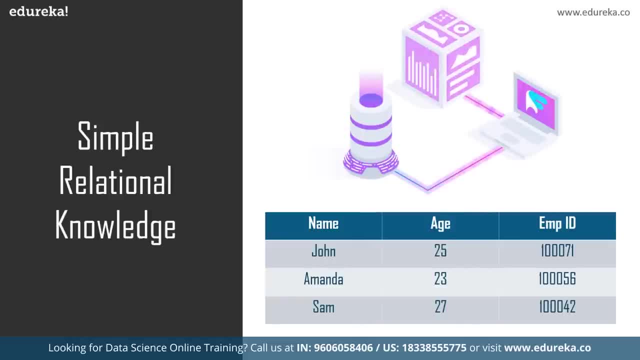 age and employee ID and we have three different names, along with their age and employee IDs. So this is how you represent a simple relational knowledge. It is the simplest way of defining. you just have to take the name age and employee ID and Define the relation. moving on. 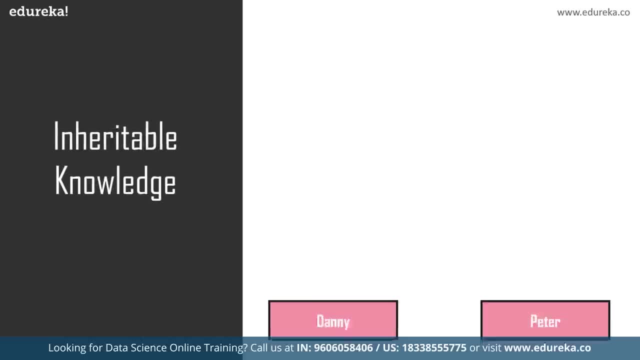 to the next approach. We have the inheritable knowledge now. in the inheritable knowledge approach, all data must be stored into hierarchy of classes and should be arranged in a generalized form or a hierarchical manner. Also, this approach contains inheritable knowledge which shows a relation between instance and class. 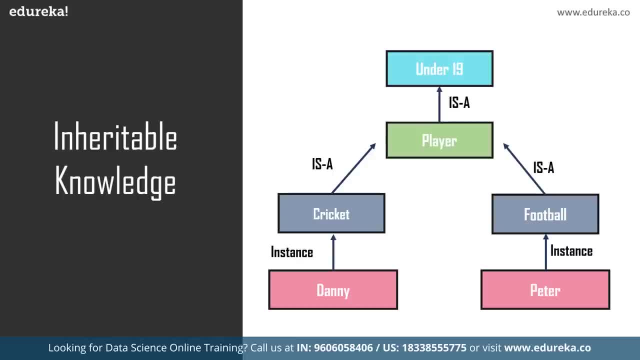 and it is called the instance relation. now, in this approach, objects and values are represented in boxed nodes. So here you can see the example where we have two different players, Danny and Peter, who plays two different games such as cricket and football, but they both are known as players.